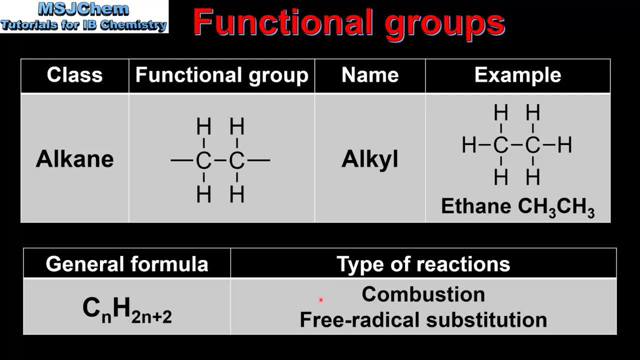 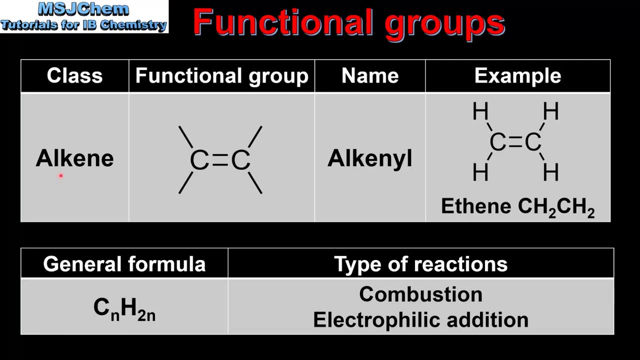 Alkanes undergo combustion reactions and free radical substitution reactions. Both these kinds of reactions are covered in more detail in later videos. The next example we look at is the alkenes. Alkenes are unsaturated hydrocarbons. The class name is alkene and the functional group 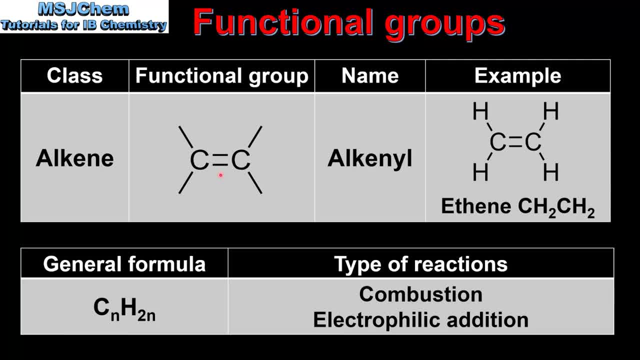 name is alkyl. The functional group is a carbon to carbon double bond. On the right we have an example of an alkene with two carbon atoms, which is ethane. The general formula for the alkenes is CnH2n, and the type of reactions that 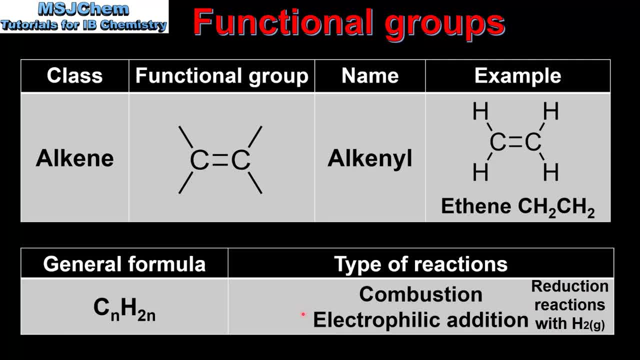 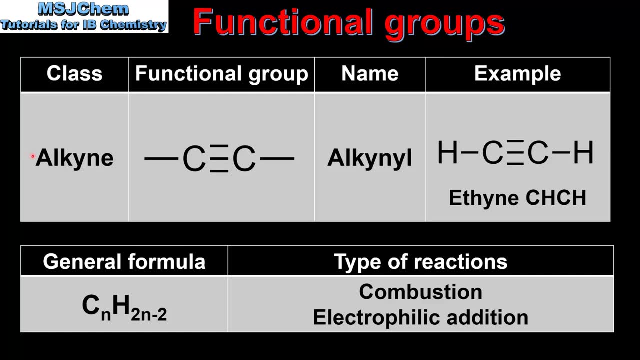 alkenes undergo are combustion reactions and electrophilic addition reactions. Alkenes can also undergo reduction reactions to produce alkanes. Next we look at the alkynes. Like the alkenes, the alkenes are unsaturated hydrocarbons. 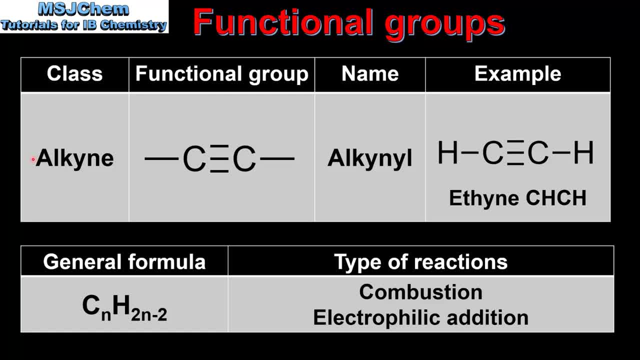 The class name is alkyne and the functional group name is alkynyl. The functional group is a carbon to carbon triple bond. An example of an alkyne is ethane, which we can see here on the right. The general formula for the alkenes is CnH2n minus 2.. Like the alkenes, alkenes undergo combustion reactions and free radical substitution reactions. Both these reactions are covered in more detail in later videos. On the right we have an example of an alkene with two carbon atoms, which is ethane. The general formula for the alkenes is CnH2n and the 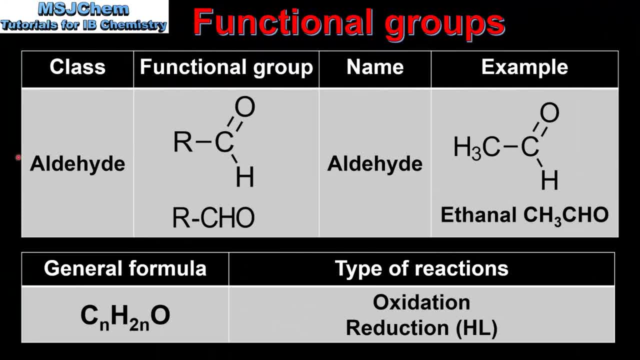 type of reactions that alkenes undergo are combustion reactions and electrophilic addition reactions. Next we look at aldehydes. The aldehyde functional group is a carbon atom that has a double bond to an oxygen atom and a single bond to a hydrogen atom. The carbon to oxygen bond is known as 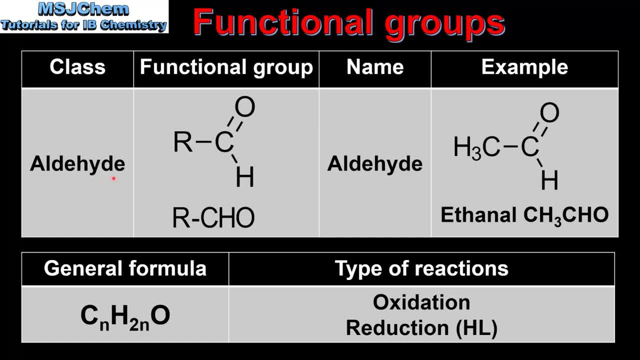 a carbonyl group. The name aldehyde is the class name as well as the name of the functional group. On the right we have an example which is ethanol. Note that in the condensed structural formula the aldehyde group is written as C-H-O, The general formula for the aldehydes. 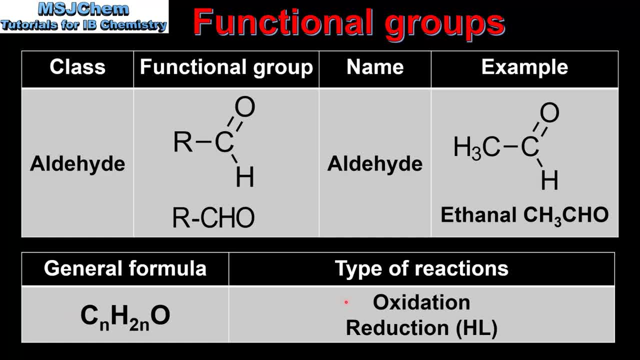 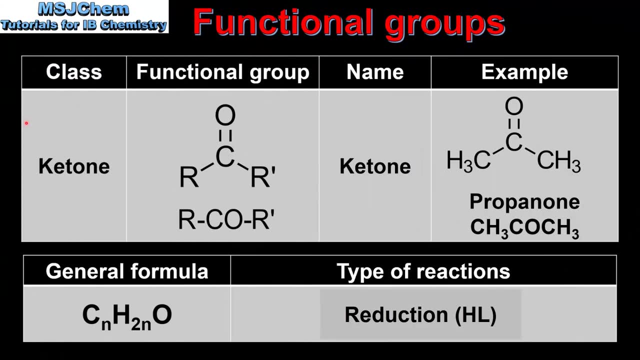 is CnH2nO. Aldehydes undergo oxidation reactions to form carboxylic acids. They can also undergo reduction reactions to form primary alcohols. This is only covered in the higher level syllabus. Next we have the ketones. The ketone functional group is a carbon atom that has a double bond. 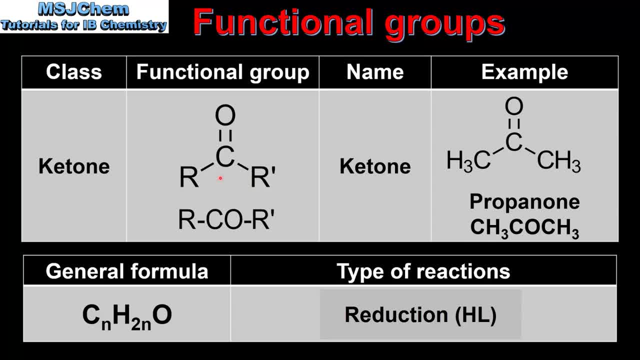 to an oxygen atom, which is also bonded to two alkyl groups. These alkyl groups are represented by the letter R, which can be the same or different. Like the aldehydes, ketones have a carbonyl group, which is a carbon double bonded to an oxygen atom. Both the class name and the functional. 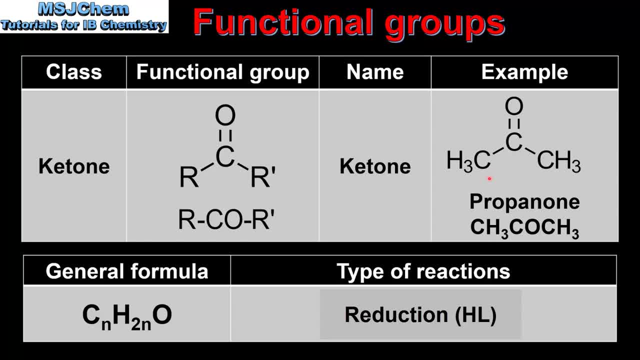 group name is ketone. On the right we have an example of a ketone which is propanone. This is the first member of the ketone homologous series. The general formula of the ketones is CnH2nO. Ketones can be reduced to form secondary alcohols. 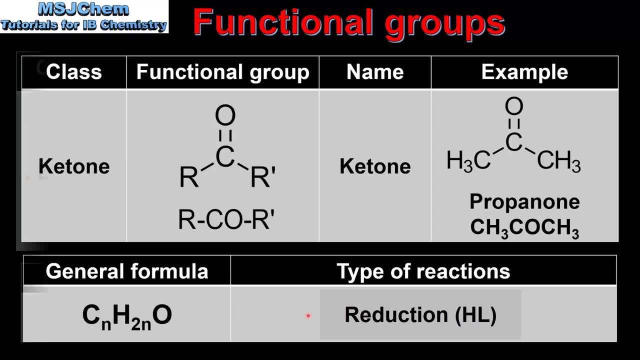 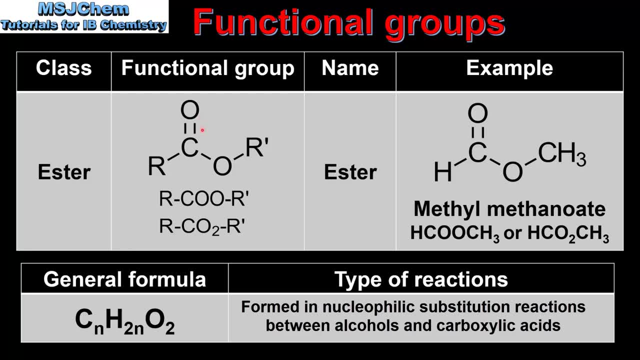 This is only covered in the higher level syllabus. Next we look at esters. The ester functional group has a carbon atom with a double bond to an oxygen and a single bond to another oxygen. Both the carbon atom and this oxygen atom are bonded to alkyl groups. The alkyl groups can be the same or different. 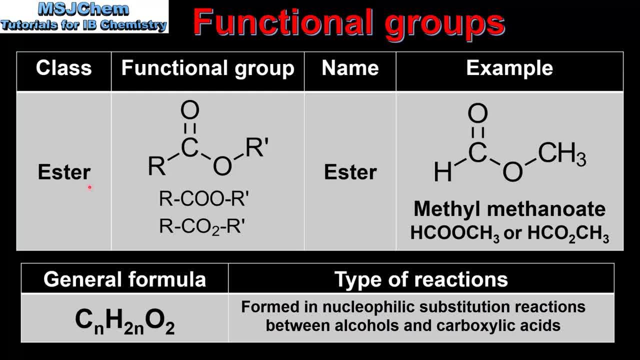 The class and functional group name is ester. Here we have an example of an ester which is methyl methanoate. Note: the condensed structural formula can be written in two different ways. The general formula for an ester is CNH2NO2.. Esters are formed in the reaction between an. 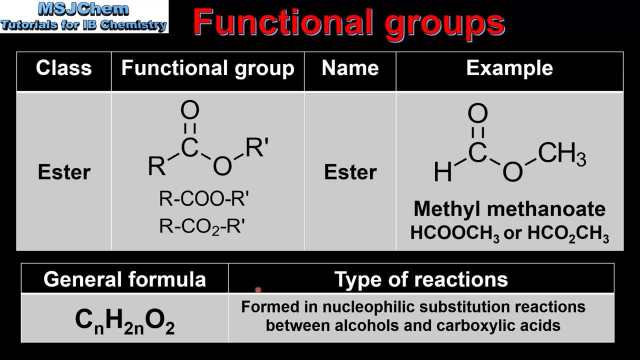 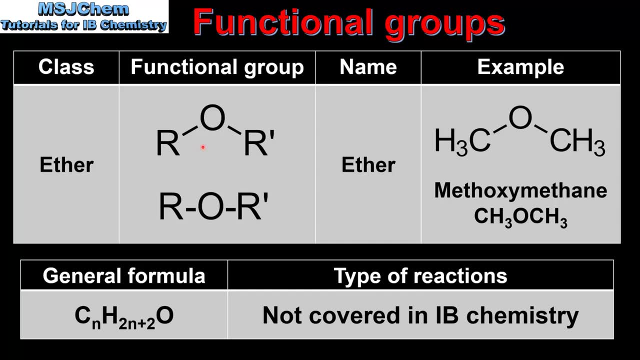 alcohol and a carboxylic acid. The reactions of esters are not required in IB chemistry, Although they can undergo hydrolysis reactions to form an alcohol and carboxylic acid. Next we look at ethers. The ether functional group is an oxygen atom bonded to two alkyl groups. 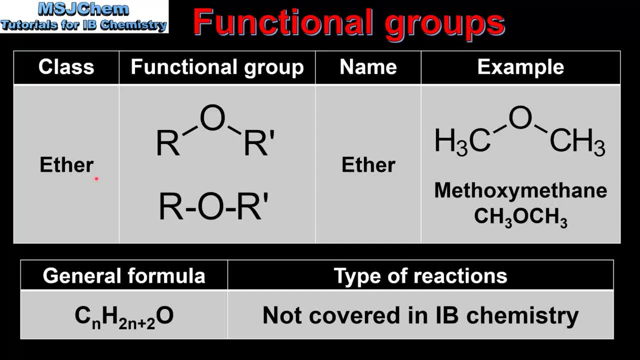 which can be the same or different. The class and functional group name is ether. Here we have an example of an ether which is methoximethane. The general formula of an ether is CNH2N2O2.. The reactions of ethers are not covered in IB chemistry. 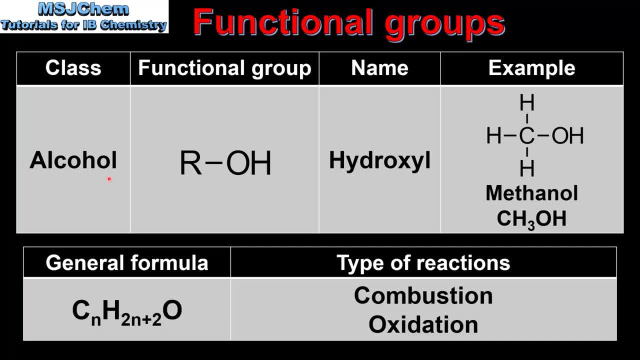 Next we have the alcohols. The class name is alcohol, but the functional group name is hydroxyl. A hydroxyl group is an oxygen bonded to a hydrogen atom. Here we have an example which is methanol. The general formula for the alcohols is CNH2N2O2.. Alcohols undergo combustion and oxidation. 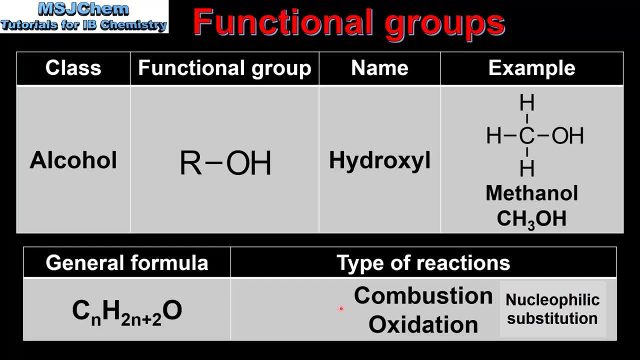 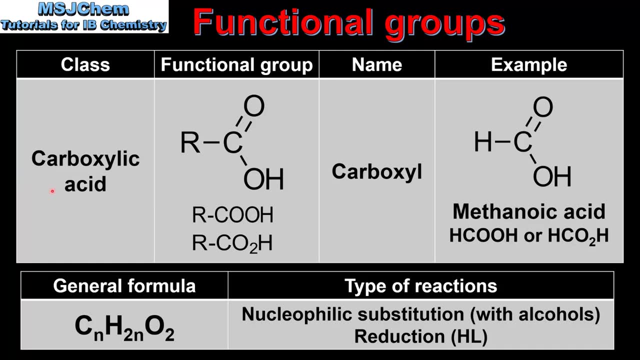 reactions. They can also undergo nucleophilic substitution reactions with carboxylic acids to form esters. These are covered in more detail in later videos. Next we have the carboxylic acids. The class name is carboxylic acid and the functional group name is carboxyl. 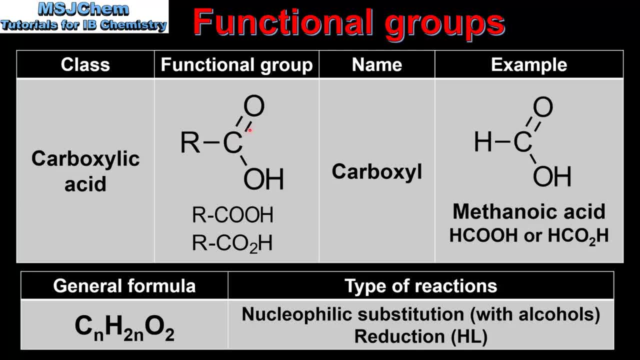 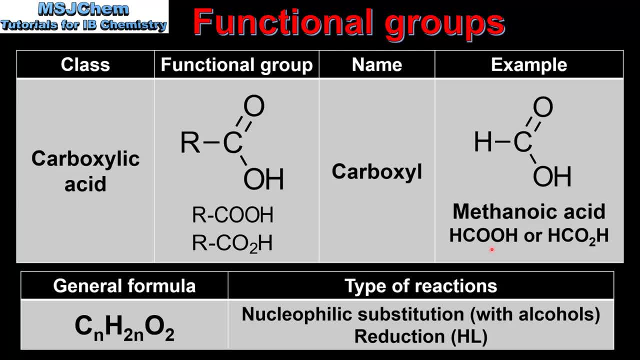 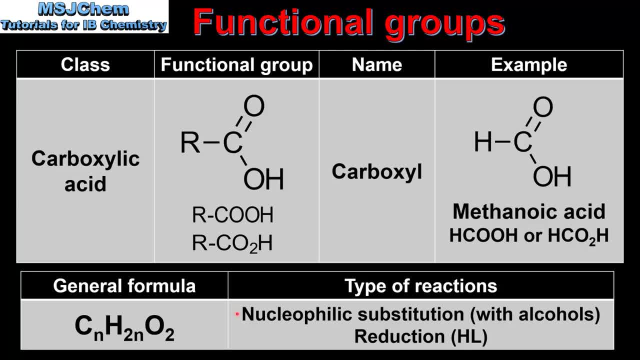 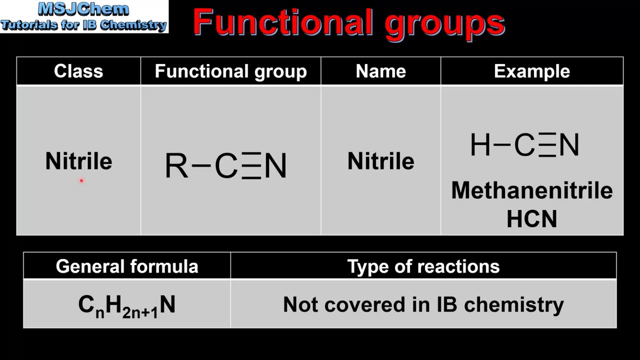 Carboxylic acids undergo nucleophilic substitution reactions with alcohols to produce esters. They also undergo reduction reactions which are covered in the higher level syllabus. Next we have the nitriles. The class name and functional group name are both nitrile. 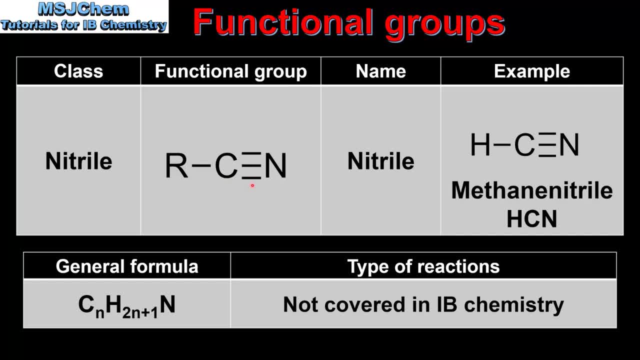 The nitrile functional group is a carboneum which, in this case, is a carbon atom, a carbon atom with a triple bond to a nitrogen atom. Here we have an example which is methane nitrile. The general formula is CnH2n plus 1n. The reactions of the nitriles are not covered in IB. 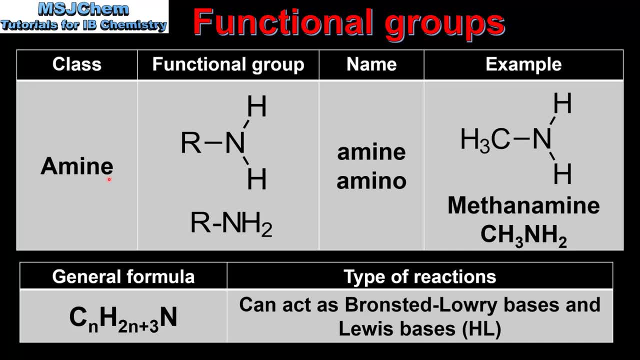 chemistry. Next we look at amines. The class name is amine. the functional group name can be amine or amino. The amine functional group is a nitrogen atom bonded to an alkyl group which is also bonded to two other hydrogens. The hydrogen atoms can also be replaced by alkyl groups. 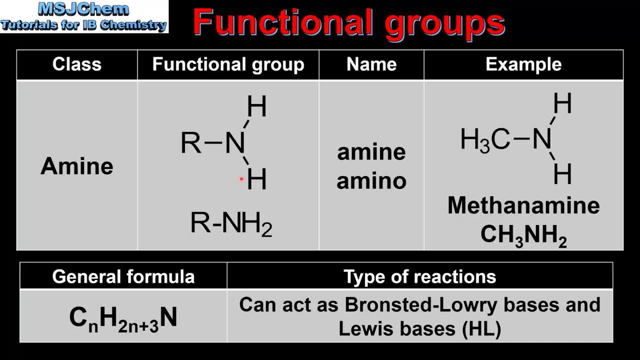 depending on if the amine is primary, secondary or tertiary. An example is methane amine, which is a primary amine. The general formula is CnH2n plus 3n. Amines can act as Bronson-Lowry bases. 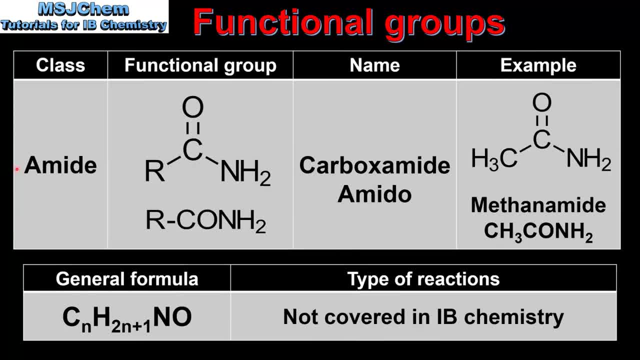 and Lewis bases. Next we have amides. The class name is amide and the functional group name is CnH2n plus 3n. Next we have amides. The class name is amide. the functional group name is is either carboxamide or amido. A carboxamide functional group is a carbon atom with a double